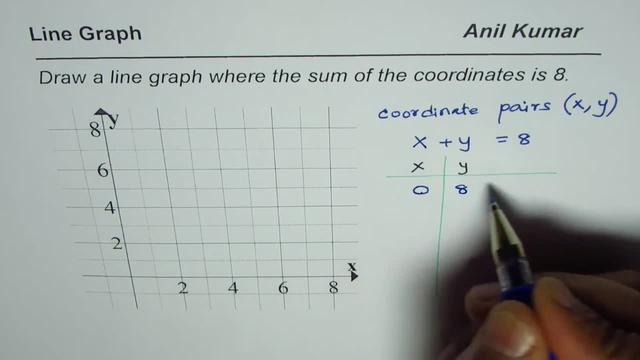 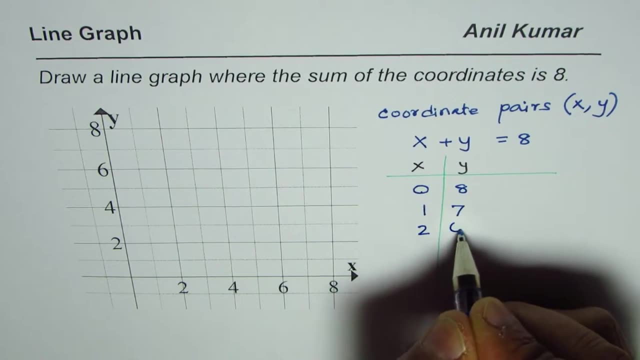 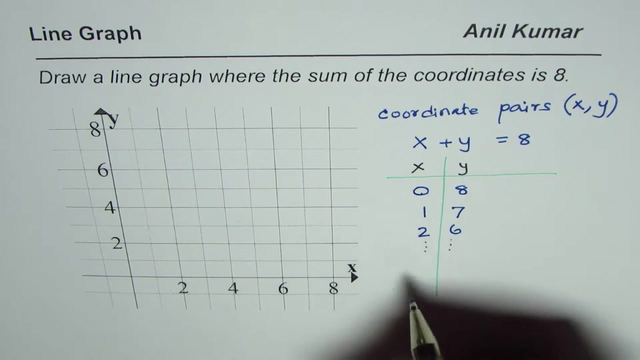 0 plus what is 8?? 0 plus 8 is 8, correct, okay, How about 1?? 1 plus 7 is 8, right, 2, 2 plus 6 is 8.. So likewise you can write many values, right Now 8,. let me write. 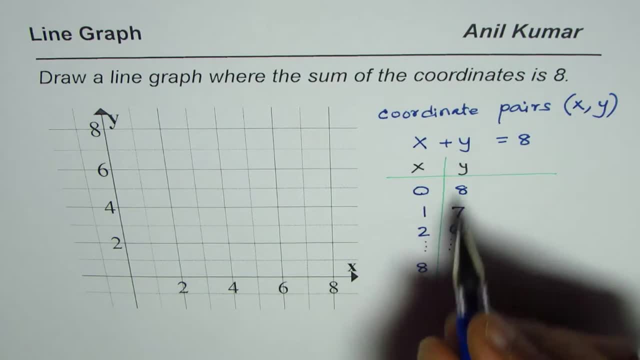 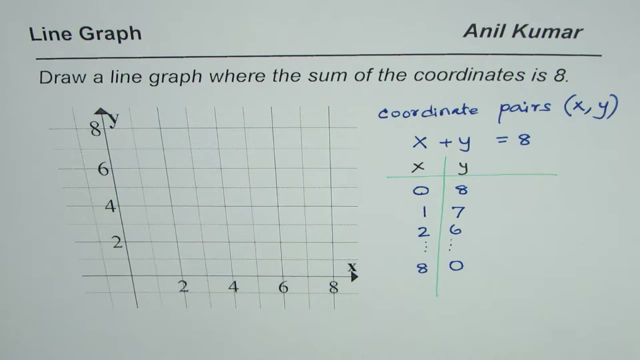 x as, let us say, 8 itself. Then 8 plus 0 is 8.. So these are some points which we can plot and join them using a straight line. Remember to draw a line. you need how many points? 2. 3 is good, 4 is even better. 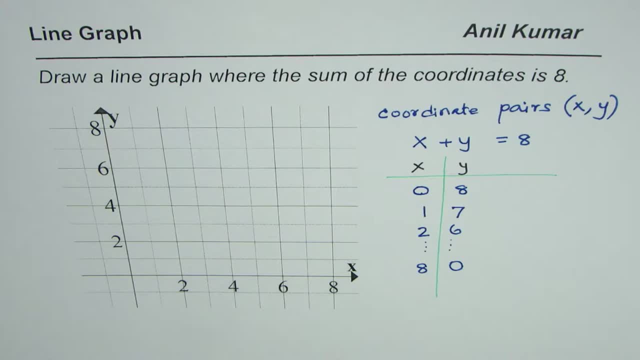 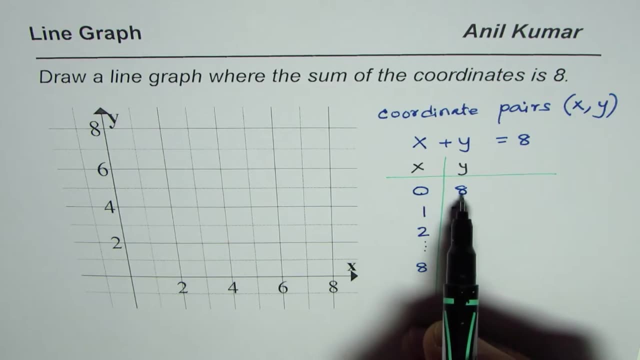 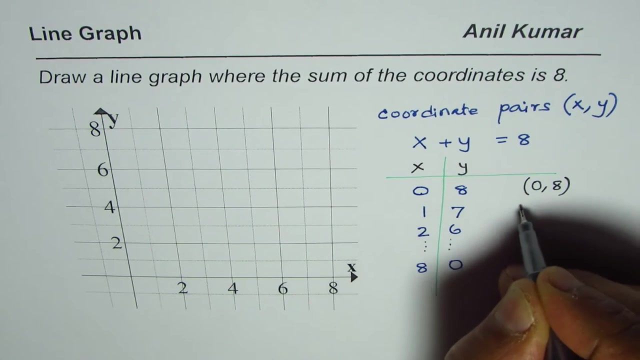 right. So now, in this case, we already have 4 points. Let us draw a line using these 4 points: x, 0. y, 0. y, 0, 8.. So that really means that the coordinates are 0 and 8, right. 1, 7 means 1 and 7, 2,. 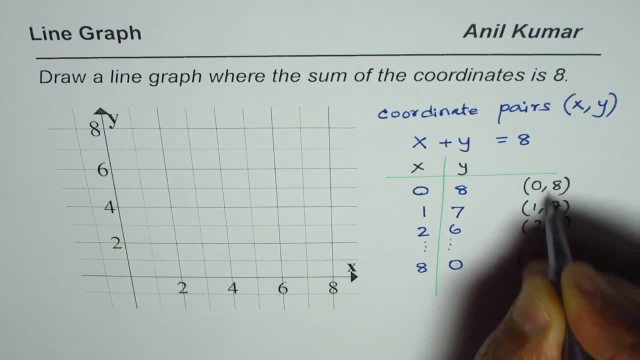 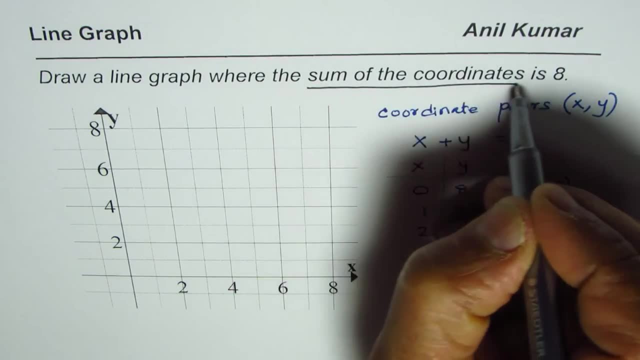 6,, and then we have 8, 0.. So these are the coordinate pairs. When you add them, you always get 8, and that's what we mean by saying sum of the coordinates is 8, correct? So let's. plot these points: 0, 8.. So that is 0 for us. We need to have an 8.. So we need to have 1, 8, 2, 6, 7, 2, a 1. This is equal to 1, 8.. We can just draw a line if we make sure. 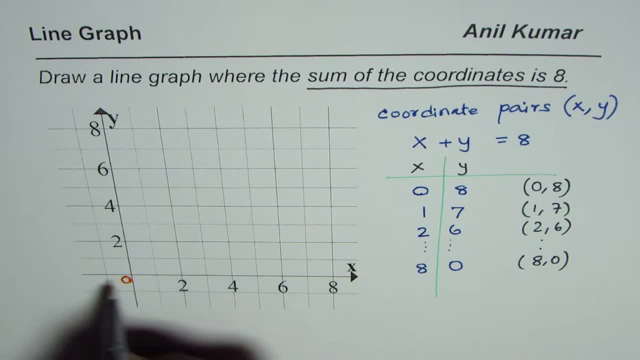 that we have an 8. We can just draw a line here, So that is equal to 1,, 8,, 9,, 13,, 12,, 13, is 0 for us. where horizontal x-axis and y vertical axis intersect, 0, 8 will mean. 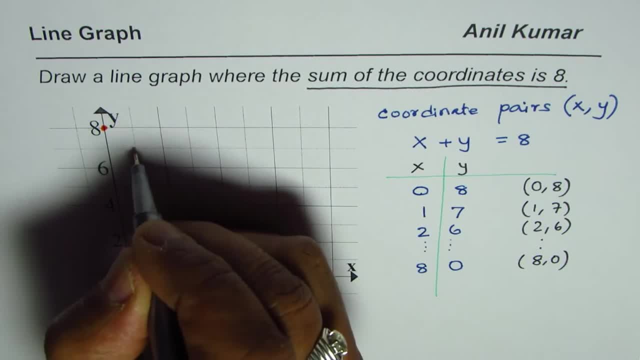 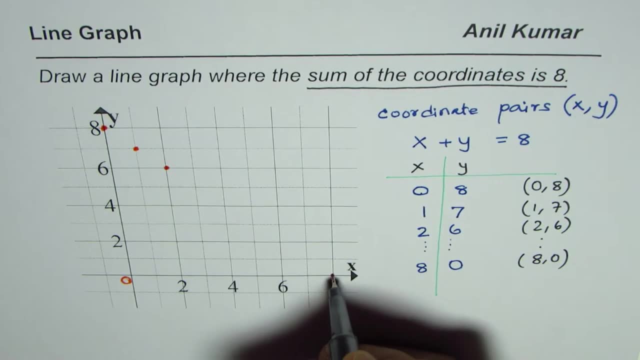 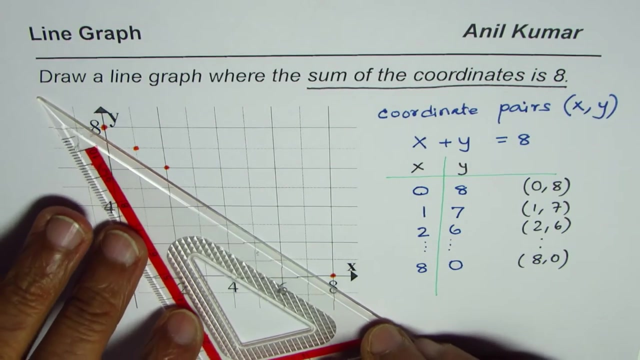 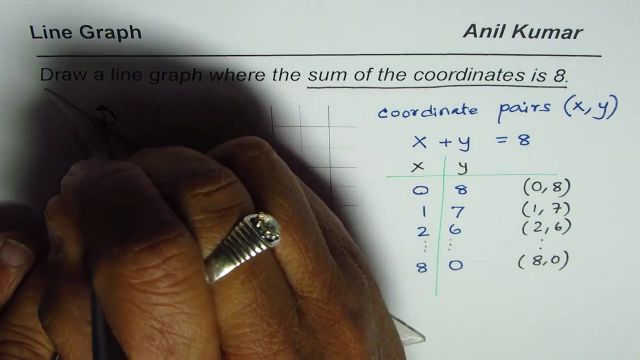 this point: 1, 7, 1 and 7 is that point, and then 2, 6 for 2, 6, 8, 0, right? so these are the points which we can join with a straight line. there you go so. so we can just draw a line like this, so that becomes the line: 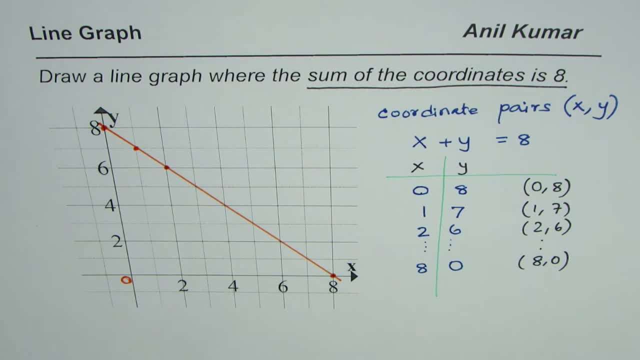 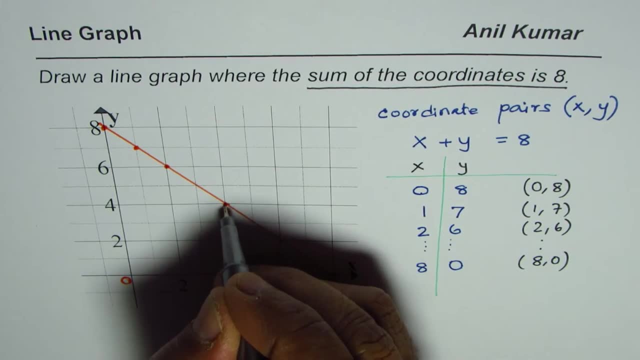 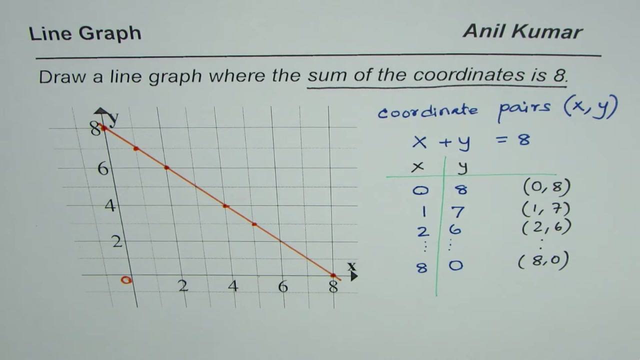 a straight line joining these points. there are many other points which you can find the coordinates like 4, 4, right. 4 plus 4 is also 8, so you can test it out. even other points, 5 and 3: when you add them it is going to give you 8. so 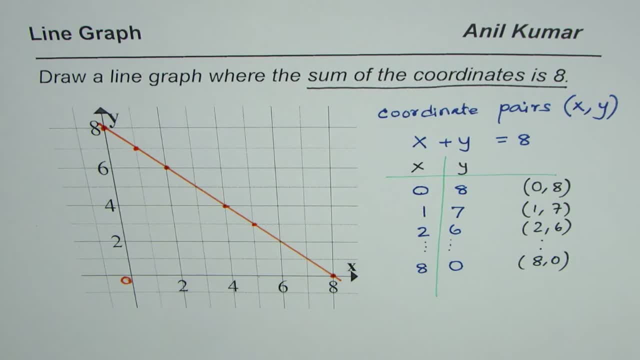 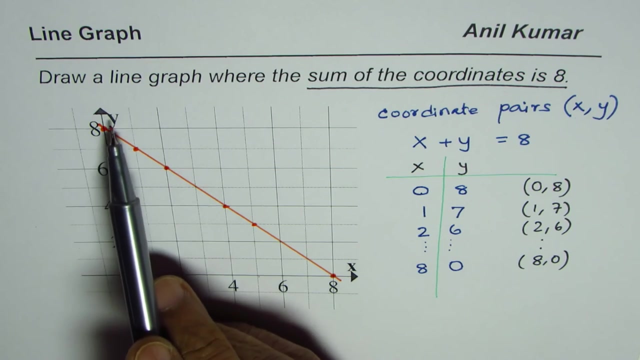 that is the line which is required. I hope you understand how we can do such questions. now there is a question for you. you need to describe the line itself. so try to describe the line. is it going upwards or downwards? is the line value values y as X increases? what happens to y? that is, 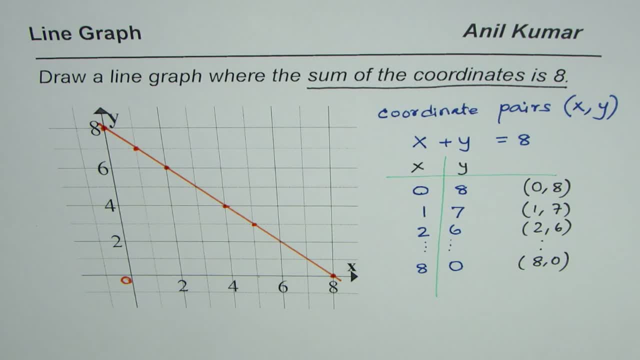 these are the things in which you can express or describe a line. so try to describe the line as an additional exercise to this video. I hope that should help you to understand the concepts. thank you and all the best. 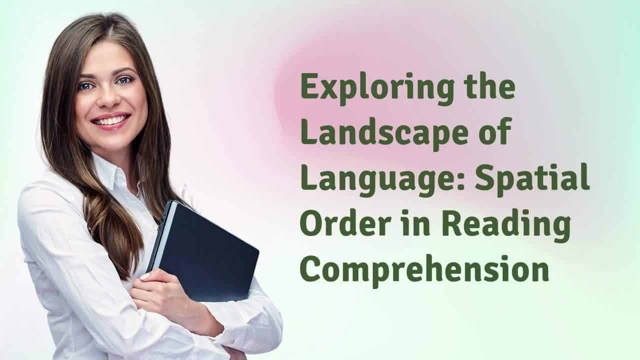 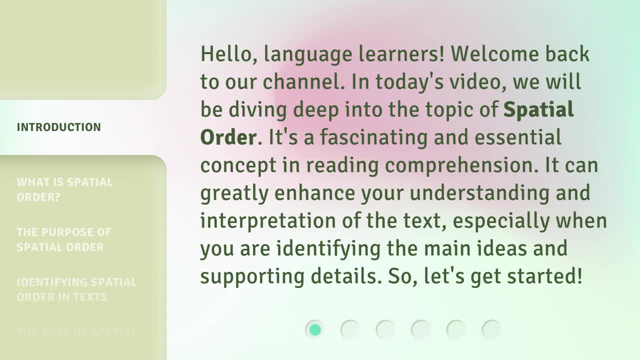 Exploring the Landscape of Language, Spatial Order and Reading Comprehension. Hello language learners, Welcome back to our channel. In today's video, we will be diving deep into the topic of spatial order. It's a fascinating and essential concept in reading. 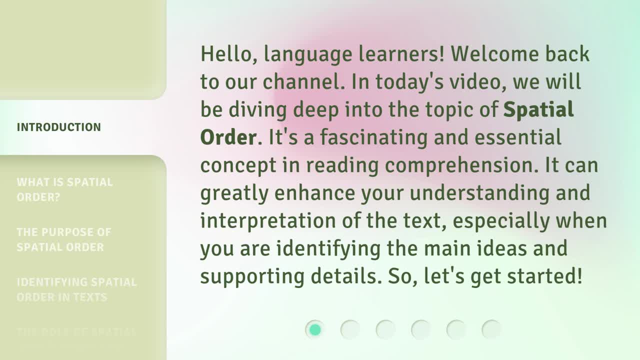 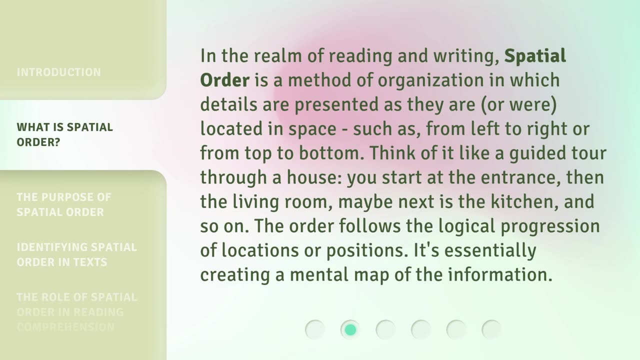 comprehension. It can greatly enhance your understanding and interpretation of the text, especially when you are identifying the main ideas and supporting details. So let's get started In the realm of reading and writing. spatial order is a method of organization in which details are presented as they are or were located in space, such as from left to right. 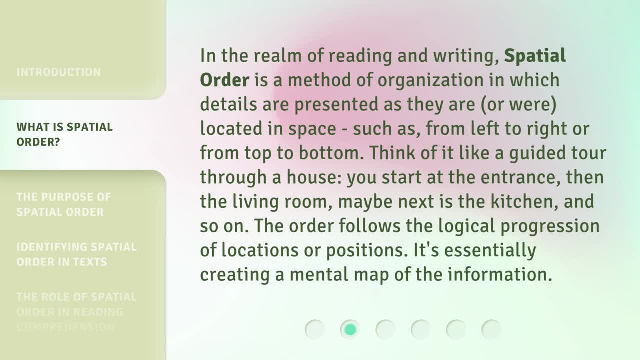 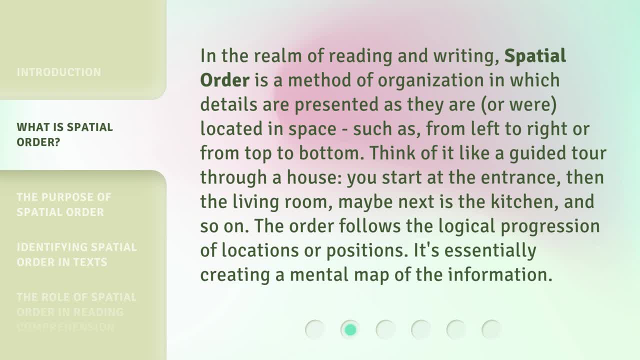 start at the entrance, then you enter the house. You start at the entrance, then you enter the living room. Maybe next is the kitchen, and so on. The order follows the logical progression of locations or positions. It's essentially creating a mental map of the information.